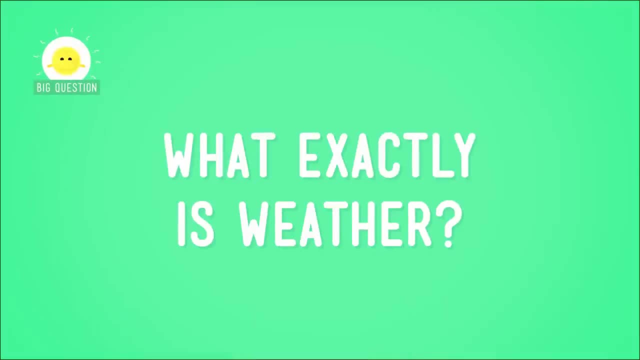 Let's start with a big and pretty basic question. What exactly is weather? 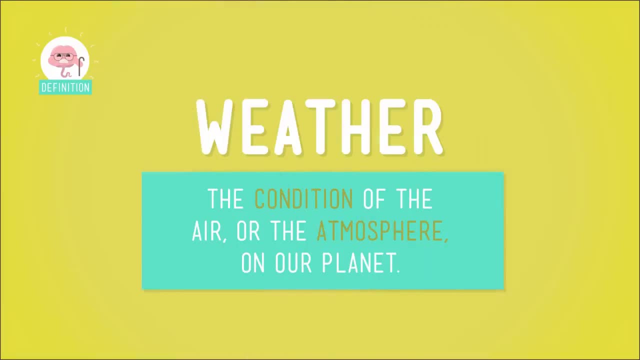 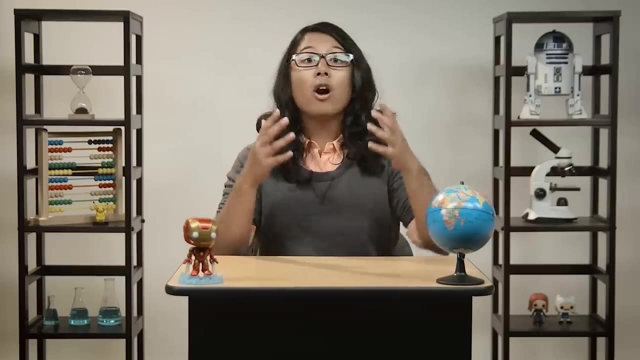 Well, weather is the condition of the air, or the atmosphere, on our planet. But the thing is, even though there's only one atmosphere on Earth, the weather isn't the same all over the world. There are many different factors that can change the atmosphere in a certain area. 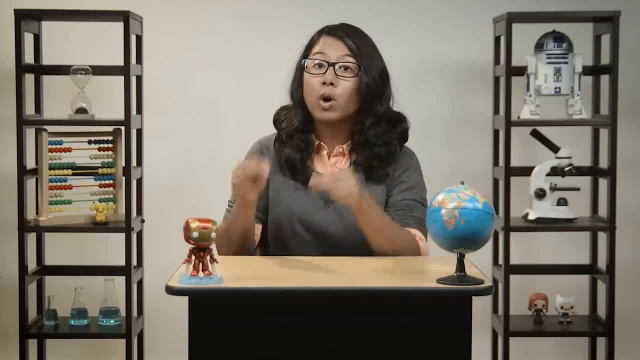 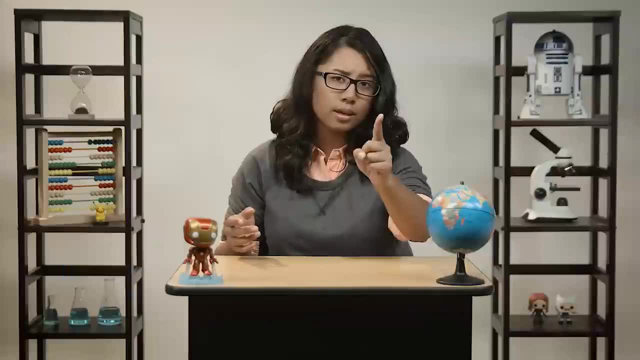 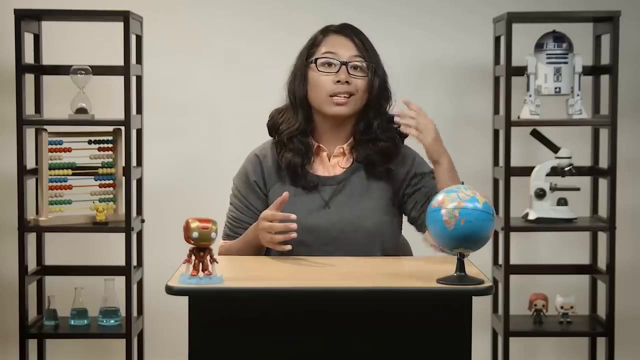 And together, they determine what the weather is like from one minute and from one place to the next. These factors include temperature, humidity, wind speed and direction, and lots of other things. But, when you're talking about the overall weather patterns from a certain region of the world, you're talking about the area's climate. 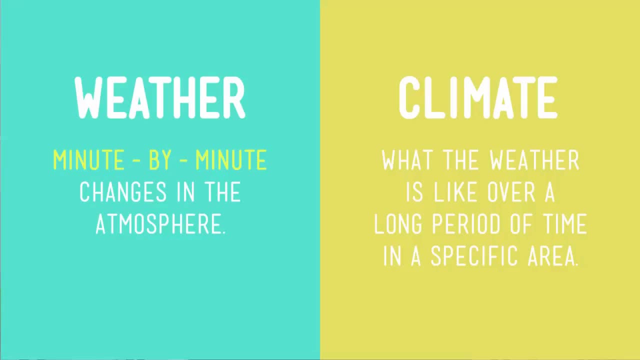 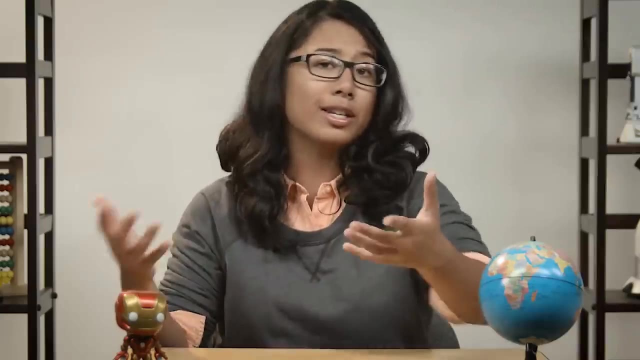 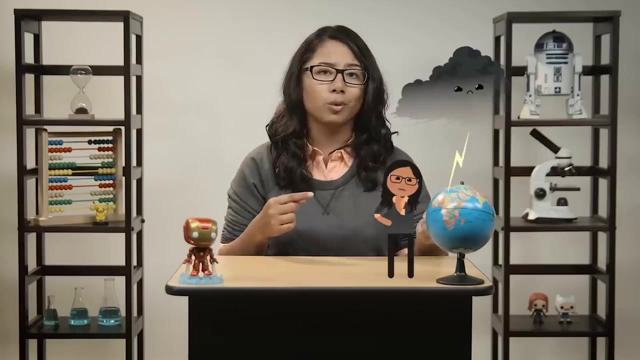 Weather is the minute-by-minute changes in the atmosphere. Climate is what the weather is like over a long period of time in a specific area. Now, the weather is constantly changing, all the time, every single day. Now, the weather is constantly changing, all the time, every single day. Think of the weather as being like that one friend of yours who could never make up their mind about what movie they want to see or what restaurant they want to go to. 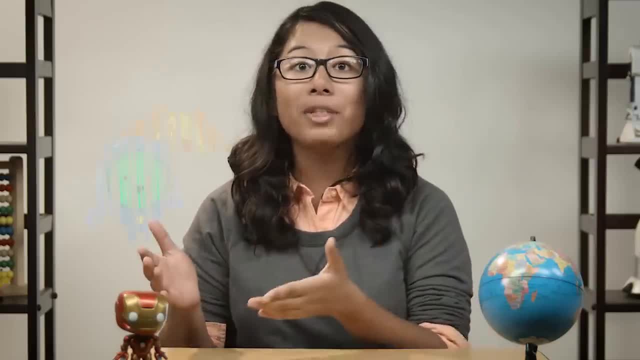 Just because it's beautiful and sunny outside when you wake up, that doesn't mean you won't need an umbrella before the day's over. 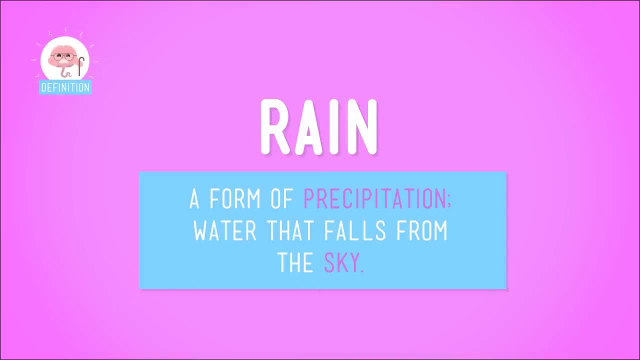 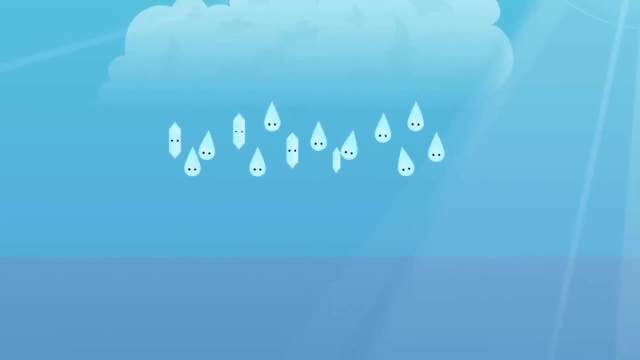 And raining is just one of the things that weather can do. Rain, of course, is just a form of precipitation, or water that falls from the sky. It happens when droplets of water in the clouds, or sometimes ice crystals, get heavy enough and fall to the ground. If they're crystals, the warm air near the ground will melt them as they fall, forming liquid rain. If they're crystals, the warm air near the ground will melt them as they fall, forming liquid rain. 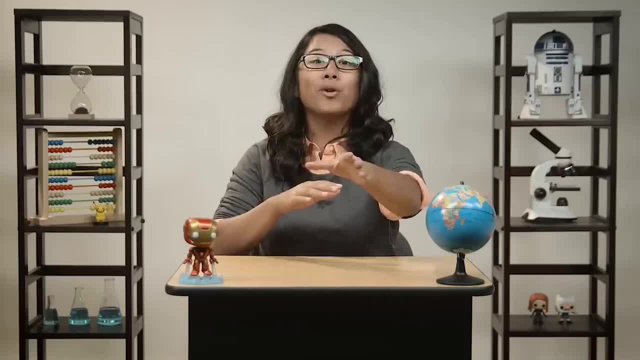 But, do you want to build a snowman? Another common form of precipitation is snow. 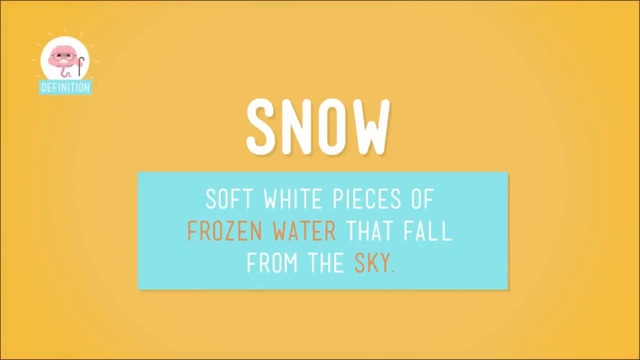 Snow is just ice crystals that don't melt into liquid water as they fall. Another snow-like form of precipitation is sleet. 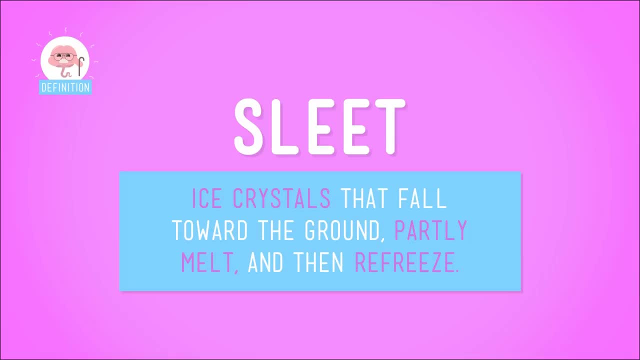 It's what happens when ice crystals fall toward the ground, partly melt, and then refreeze again. 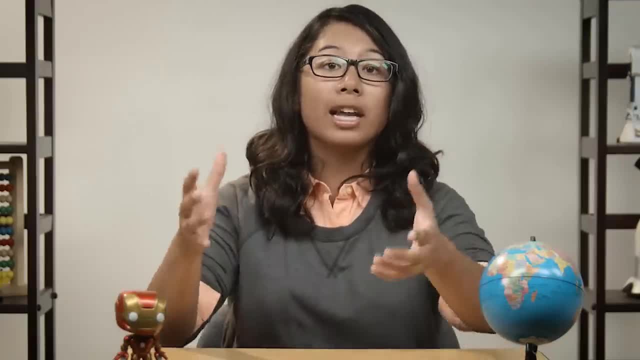 But other kinds of weather can be way more severe. And the most common kind of extreme weather is a form I'm sure you're familiar with. Thunderstorms. 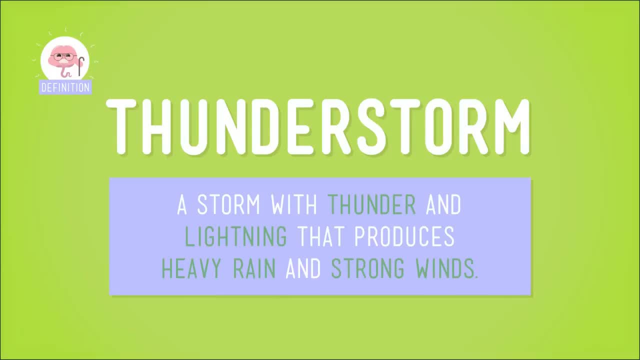 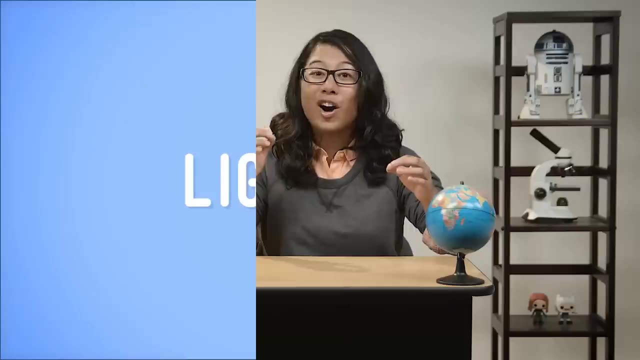 A thunderstorm can happen when strong winds make drops of water and pieces of snow. The drops of water and pieces of ice collide and break apart inside a storm. This causes electrical energy to build up, which creates a little something called lightning. 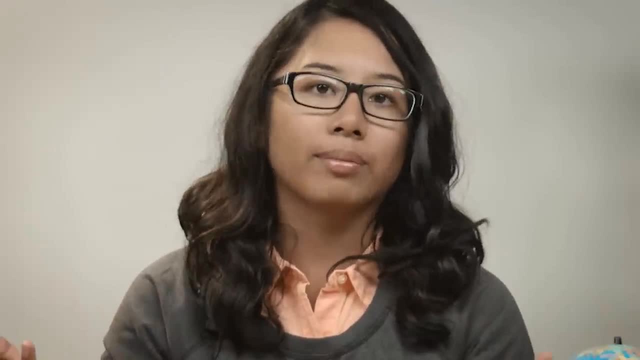 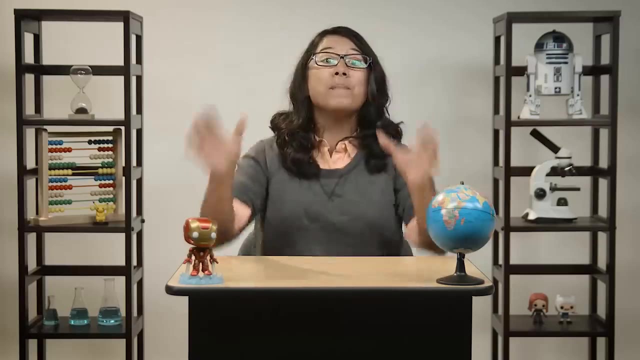 But all of this rain and snow and sleet I've been talking about, that's all just weather. And while weather can change in a few hours, a region's climate takes hundreds, thousands, even millions of years to change.